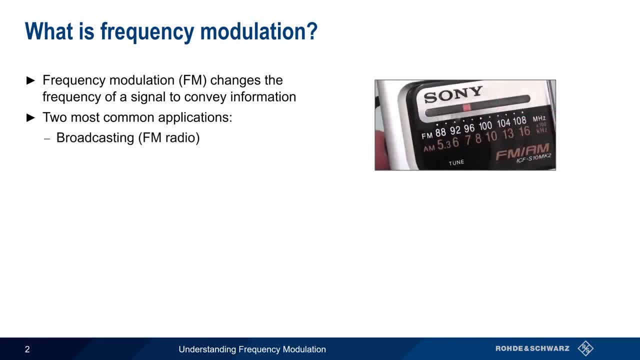 of frequency modulation are commercial FM broadcasting or FM radio and local two-way communications. Because frequency modulated signals require relatively wide bandwidths, FM is normally only used at VHF and higher frequencies, that is, at frequencies above 30 MHz. 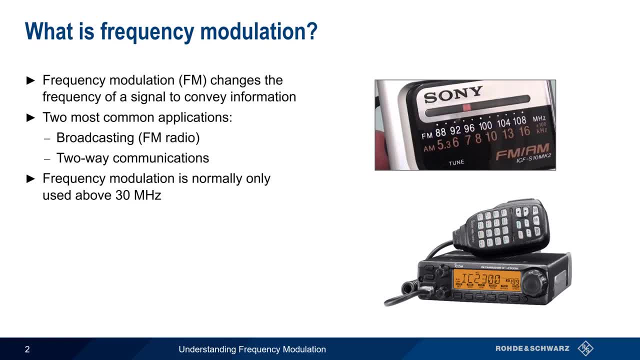 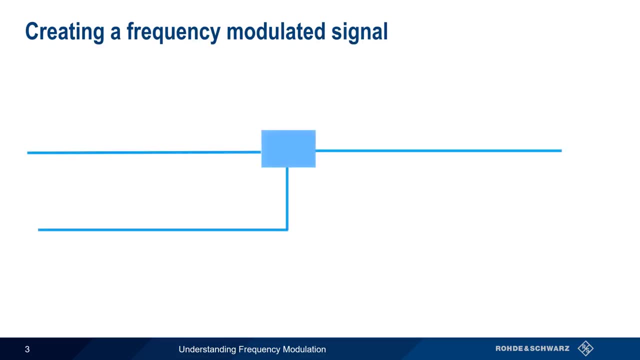 FM is almost exclusively used to transmit audio, either speech or music, and, as we'll see, one of the major advantages of FM is that it can provide both high quality and high immunity to interference fading, etc. FM signals are created using an FM modulator, the inputs to which are an unmodulated RF. 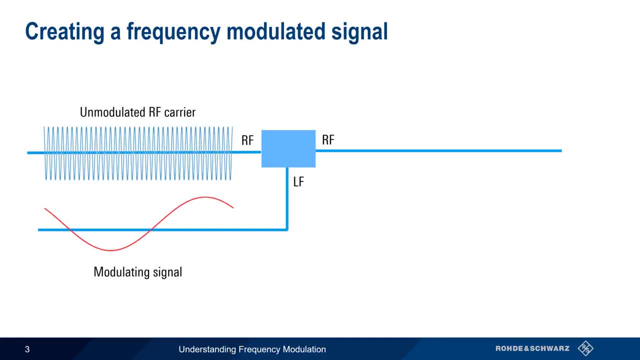 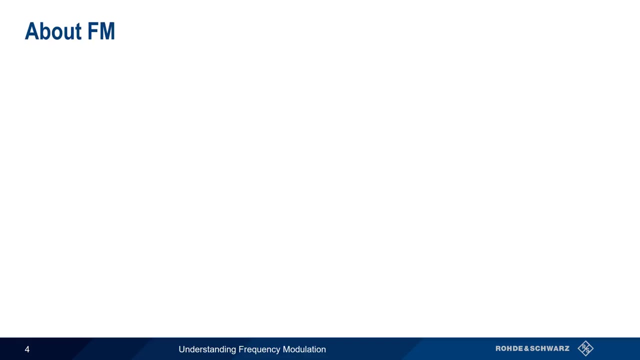 carrier and a low-frequency modulating signal. The result is a modulated RF carrier whose frequency continuously increases and decreases based on the amplitude of the signal. Frequency modulation offers quite a few advantages over other forms of analog signal modulation. Because FM transmits information as changes in frequency, it's relatively immune to changes. 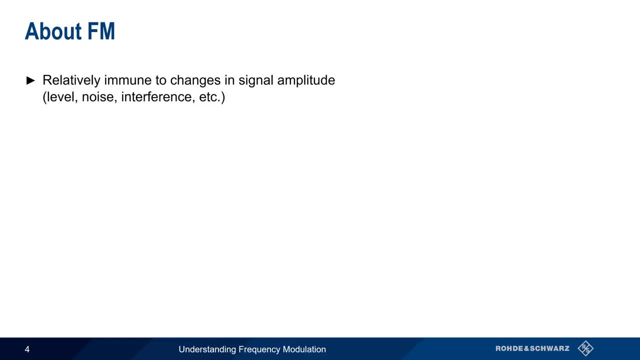 in signal amplitude, such as those caused by fluctuations in the received signal level, noise interference, etc. This makes FM a good choice for mobile or portable communications. where the RF and propagation environment may be rapidly changing, And since amplitude is not used to convey information, FM is a good choice for mobile or portable communications. 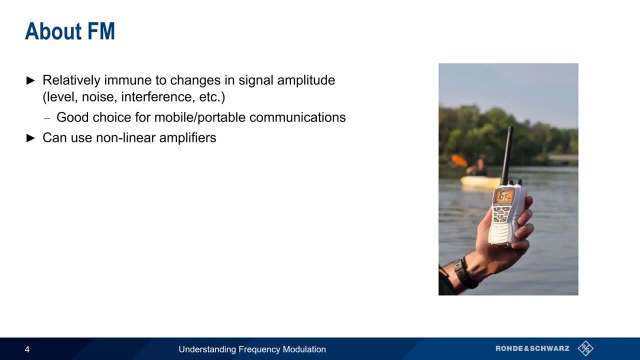 FM can also use so-called nonlinear amplifiers, whose efficiency provides an advantage in terms of power consumption and thus longer battery life. Again, this is important for portable operation. However, FM does have a relatively poor spectral efficiency compared to other analog modulation schemes like conventional AM or single sideband, in that it requires 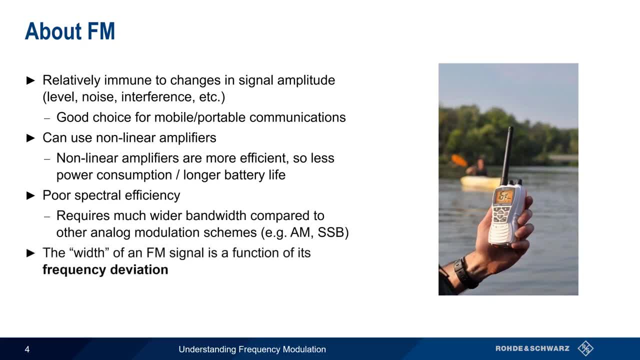 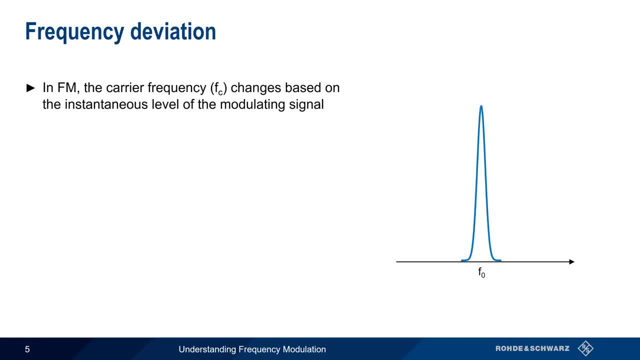 much wider bandwidths. The width of an FM signal is a function of its frequency deviation. Remember that in FM the carrier frequency- f sub c- changes based on the modulating signal. In other words, the carrier moves up and down in frequency as the modulating signal changes. 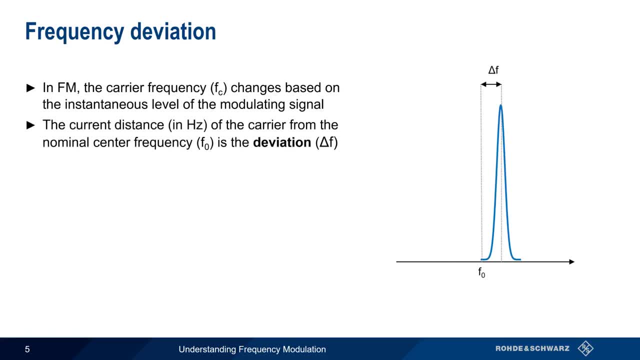 A very important concept in FM is deviation, which is the current distance in hertz of the carrier from the nominal center frequency of the signal. This deviation can be either positive or negative. For example, a deviation of 15 kHz means that the carrier is currently 15 kHz above the nominal center frequency. 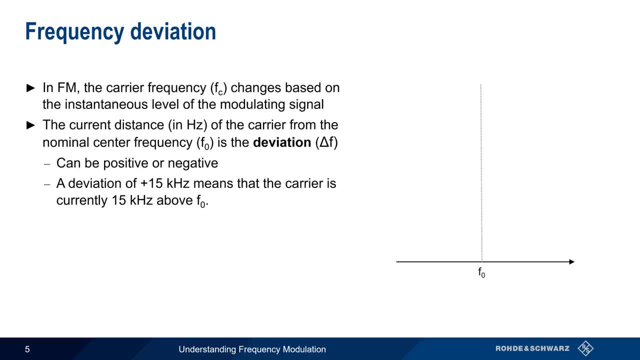 In many cases, when people talk about the deviation of an FM signal, what they really mean is the maximum deviation of the signal, that is, the maximum distance away from the center. This value is a function of the design and configuration of the transmitter. 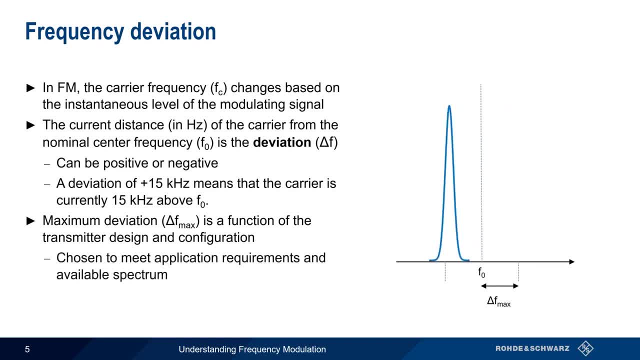 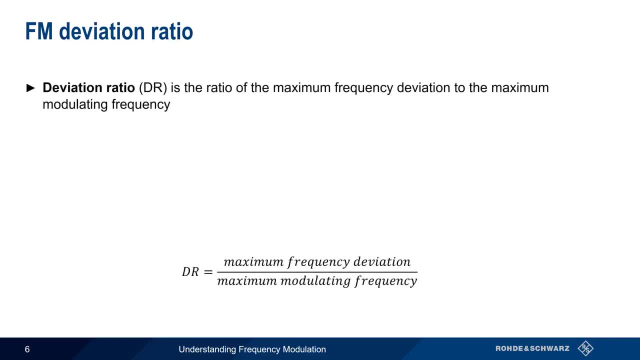 and is chosen to meet the requirements of the application and the amount of available spectrum. Deviation ratio is the ratio of the maximum frequency deviation to the maximum modulating frequency. The deviation ratio will be different depending on the application. For example, music has a relatively high maximum modulating frequency. 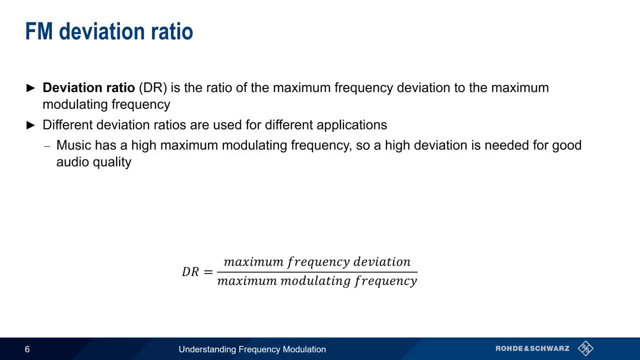 and this in turn requires a relatively high frequency deviation if we want good audio quality. On the other hand, normal human speech has a lower maximum modulating frequency, so we can use a lower deviation and still have intelligible signals. Deviation ratio is often used to group FM signals into two general categories. 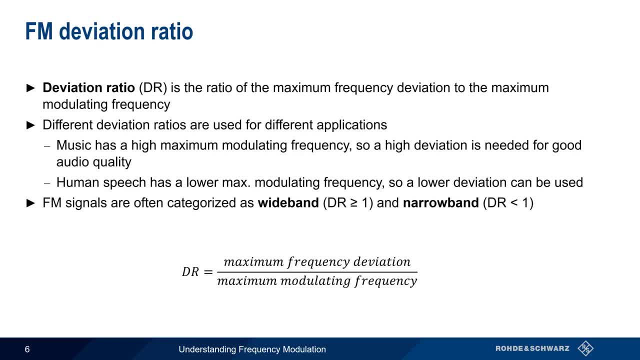 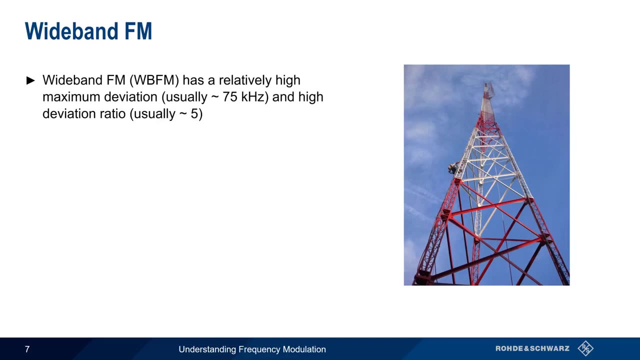 wideband FM, which has a deviation ratio of greater than 1, and narrowband FM, which has a deviation ratio of less than 1.. Let's look at the differences between these two different categories of FM. Wideband FM generally has a relatively high maximum deviation, usually 75 kHz. 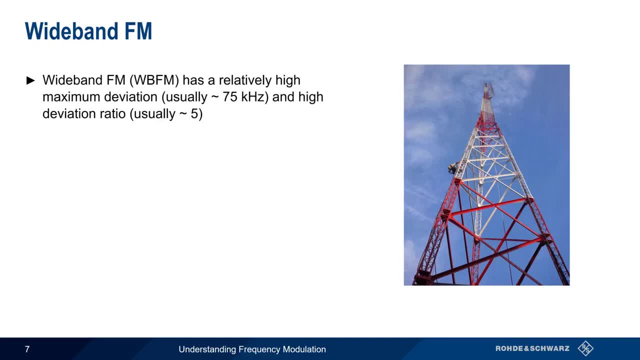 and a high deviation ratio, typically about 5.. As mentioned earlier, using a larger value for deviation provides better audio quality, especially in the case of music, but this also increases the resulting bandwidth of the FM signal. As you might expect, wideband FM is most commonly used to group FM signals into two general categories. 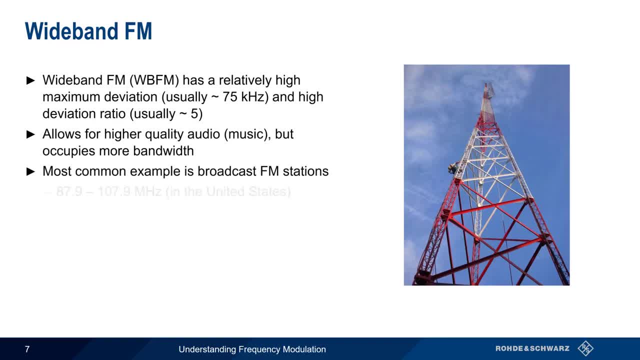 and this is often used by commercial broadcasters. In the United States. these signals can be found from 87.9 to 107.9 MHz, with station space 200 kHz apart. Narrowband FM has a much lower maximum deviation compared to wideband FM. 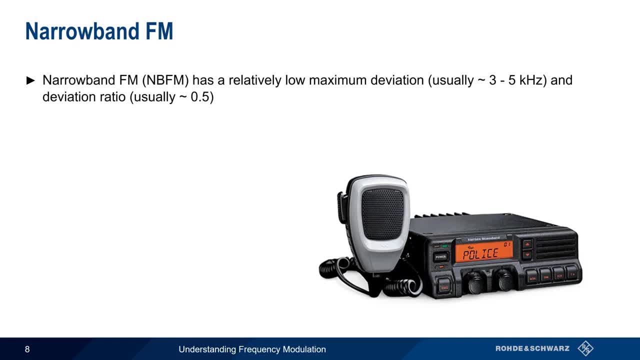 usually only 3 to 5 kHz. By definition, the deviation ratio of narrowband FM signals is always less than 1, and in practice they tend to be somewhere around 0.5,, although this can vary widely between radios, speakers and applications. 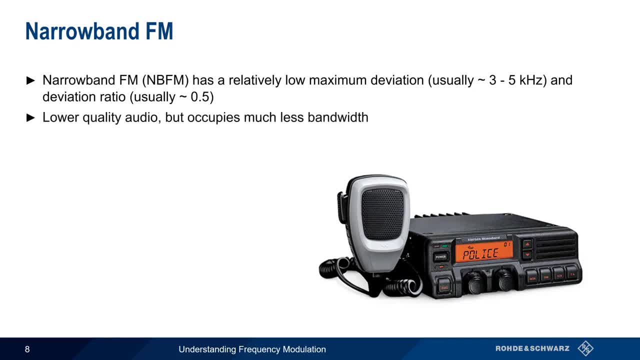 This lower deviation ratio means lower audio quality, but also a narrower signal bandwidth, and thus narrowband FM is normally used for two-way voice communications. Typical channel widths are usually 12.5 or 25 kHz, although this too can vary depending on the application.